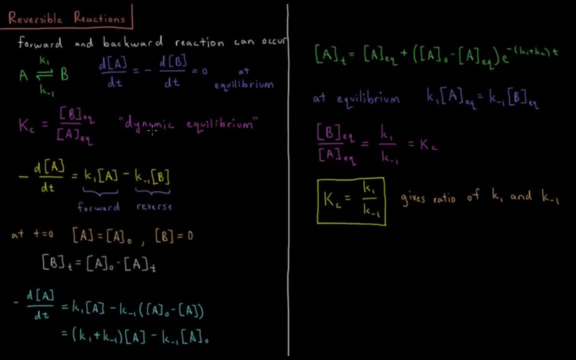 what we say is that we have achieved a dynamic equilibrium where the concentration of B divided by the concentration of A, which are going to be the equilibrium values of one another, is equal to our equilibrium constant. Okay, so when that is the case, when that's not the case, we have our rates that we can. 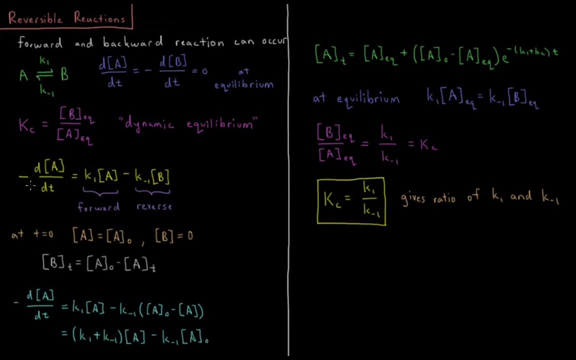 use to determine how fast those are changing. So our reaction rate minus dA dt is equal to k1 times the concentration of A. that's the forward rate constant times. the concentration of A minus k-1 times the concentration of B, our reverse reaction rate constant times. 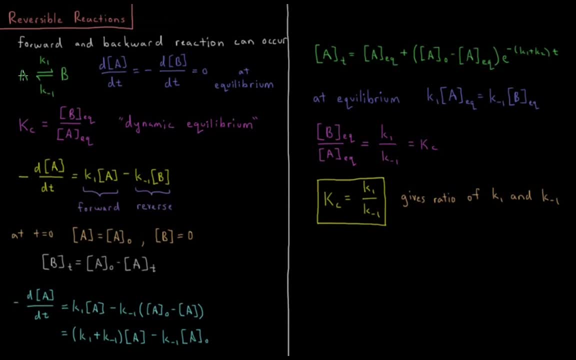 the concentration of B. Um, here we're just assuming that the reaction, the forward and reverse reaction, are first order in A and B, uh, respectively. Okay, so let's assume that at time equals zero, that the concentration of A equals A. 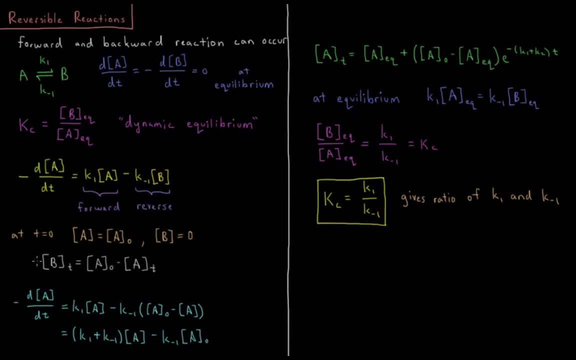 naught and the concentration of B equals zero. This means that the concentration of B as a function of time equals A naught minus A of t. So now we have minus dA. dt again equals k1 times A minus k-1 times. the concentration of B is a naught minus A. 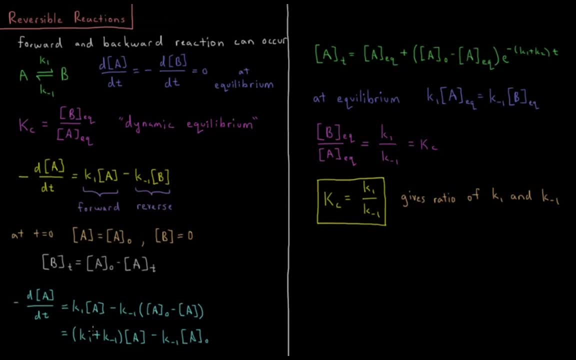 So this is equal to, if we factor things out, k1 plus k-1 times the concentration of A, minus k-1 times the concentration of A initially. So if we separate variables and integrate, what you'll get for an integrated rate law. 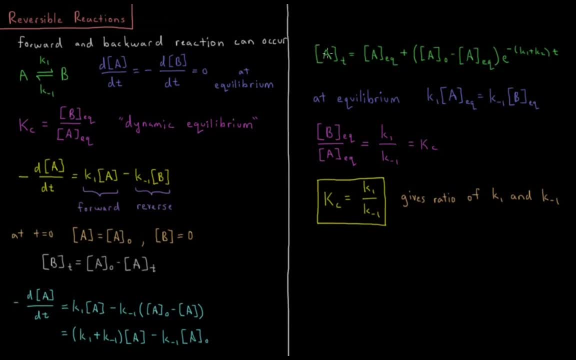 in this case is that the concentration of A this time we get is a factor of k2 times k-1, times the concentration of A, this time we get a factor of k2.. And then there's a concentration of A as a function of time is equal to the equilibrium concentration of A. 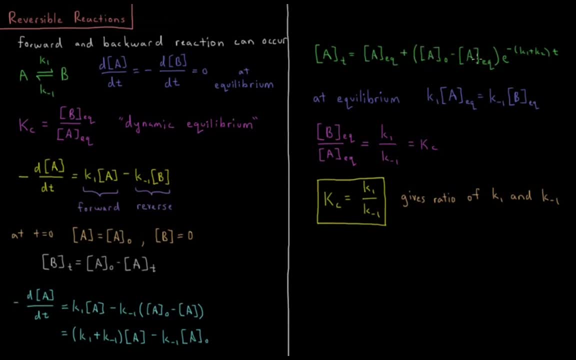 plus the initial concentration of A, minus the equilibrium concentration of A times E, to the minus K1 plus K2, or sorry, K1 plus K minus 1.. Let's fix that. There we go: K1 plus K minus 1 times T, So at equilibrium, as we saw, K1 times A, equilibrium equals K minus 1 times B.